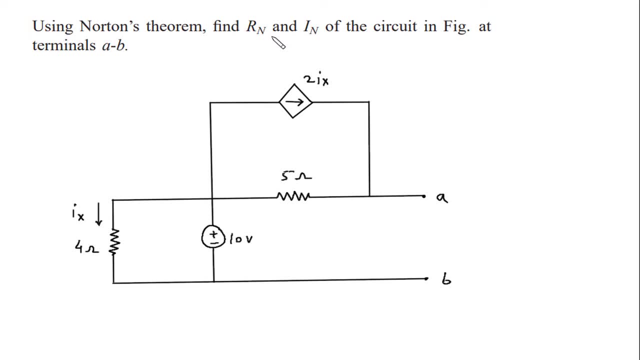 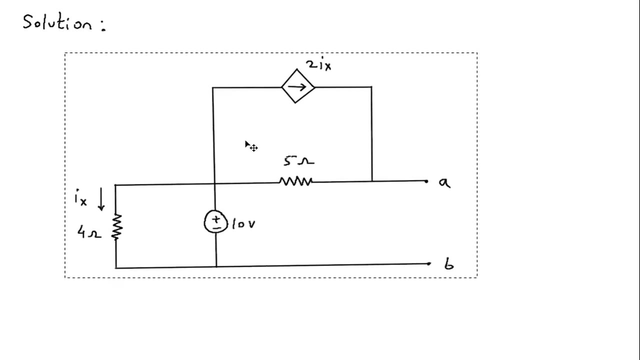 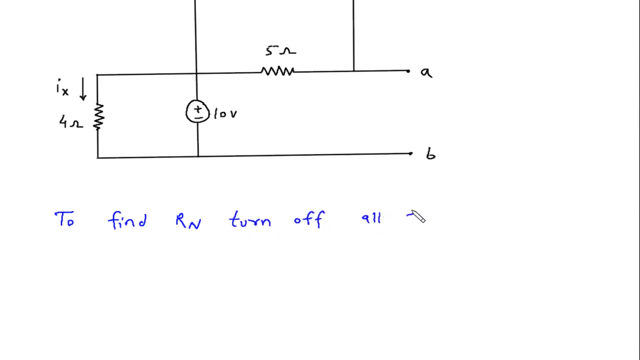 Using Norton's theorem find Rn and In of the circuit in figure at terminals a, b Solution: First of all we will redraw the circuit Now to find Rn, turn off all the independent sources. So independent source here is this is a voltage source which is independent. 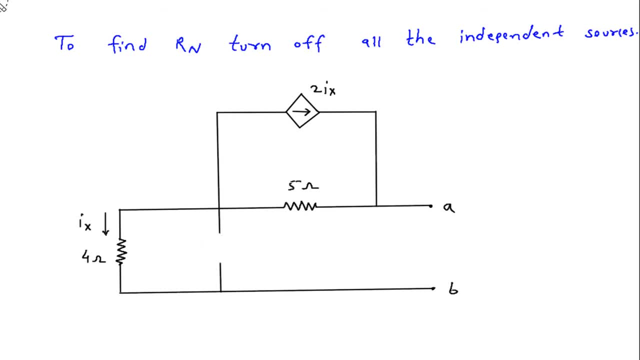 So when we turn off the independent voltage source, then that will be a short circuit. So this will be short circuited and this Ix will be equal to Ix is equal to zero, So this also will be zero. Now, when the dependent current source is zero, then that will be a open circuited. 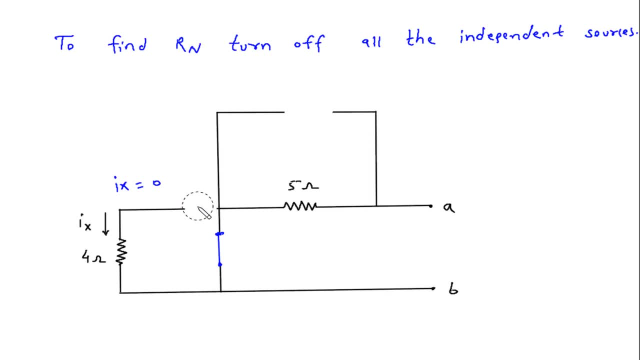 So this will be open circuited. Now to find Rn, Rn will be here. we can directly get the value of Rn or we can apply Vo, which is one volt. We can take any value here And let's say: this is Rn. 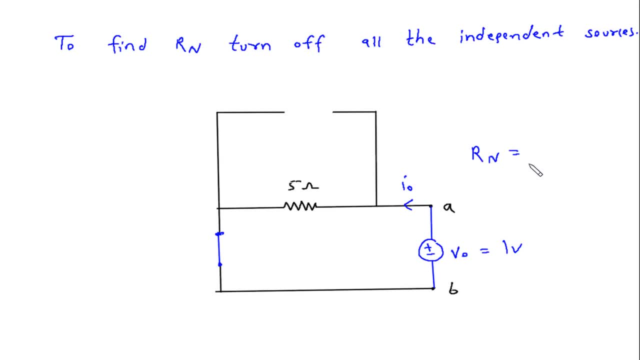 So Rn is equal to Vo, which is one volt by Io. So if we found the value of Io, then from that we can get the value of Rn. So Io will be equal to voltage, which is one by resistance, which is five. 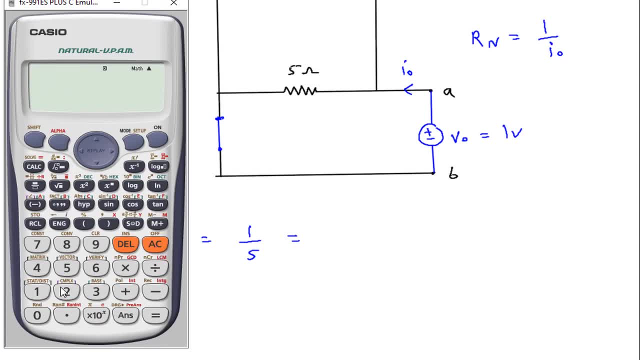 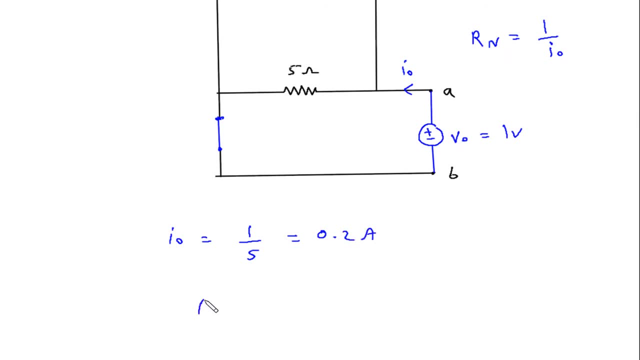 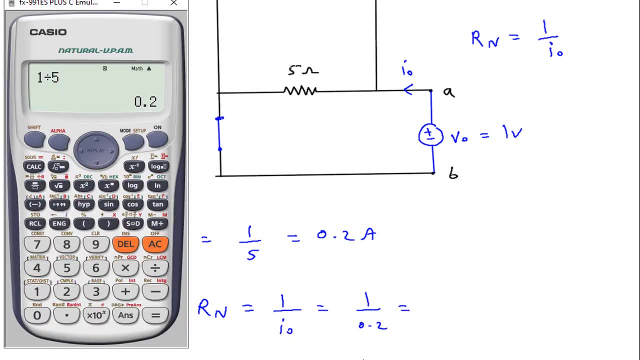 So this is one by five, One by five or zero point two, ampere. So Rn is equal to Rn is equal to one by Io. So one by zero point two is equal to one by zero point two is equal to five ohm. 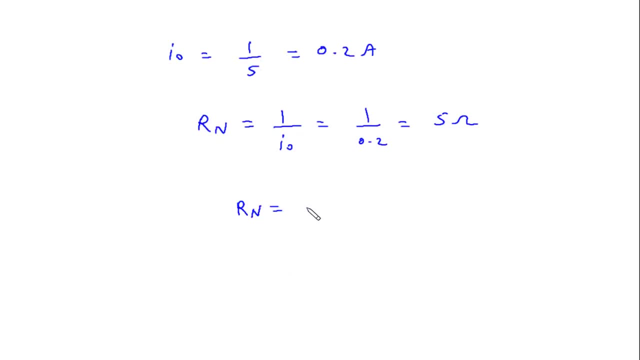 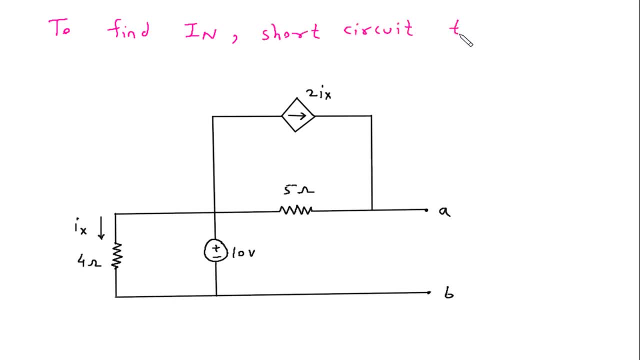 Short circuit, terminal a, b, So this will be short circuited and this will be current I? n. Now, this is short circuited, So this is short circuited And this is current V? n. this Ix will be equal to. let's say, this is ground, so Ix is equal to voltage, which is 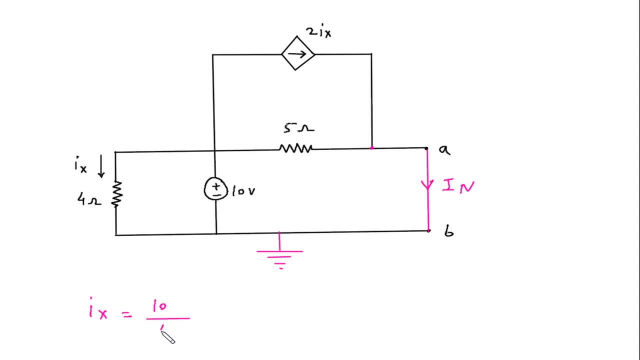 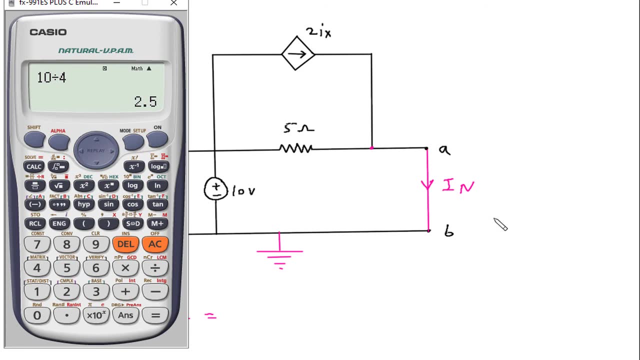 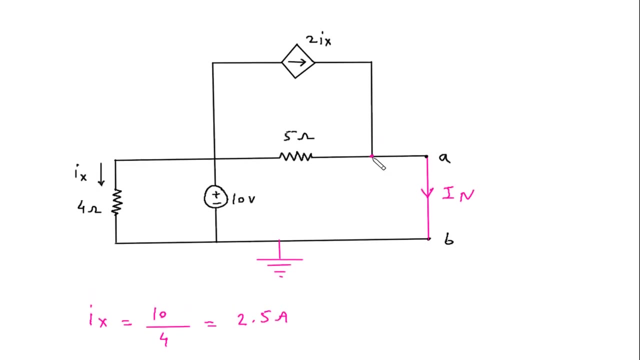 10 volt by resistance, which is 4. so this will be 10 by 4, 10 by 4, which is 2.5 ampere. 2.5 ampere is the value of Ix. now let's say this is node A. so apply KCL at, apply KCL at node. 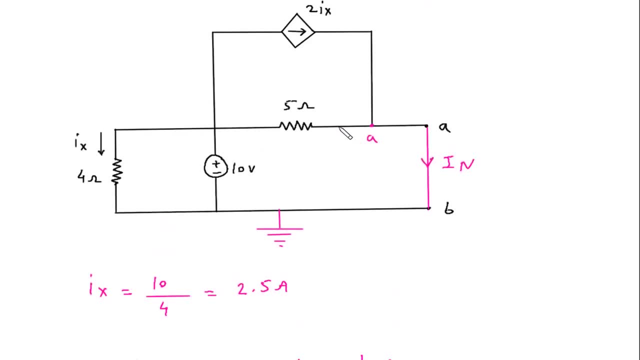 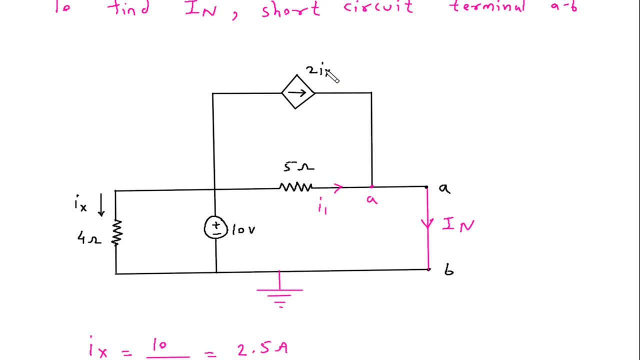 A. so let's assume this is current I1 and this is 2 Ix. so entering current at this node is 2 Ix plus I1, 2 Ix plus I1.. Okay, Okay, Okay Okay. I1 is equal to living current is IN. IN is the living current now 2 into Ix, is Ix is. 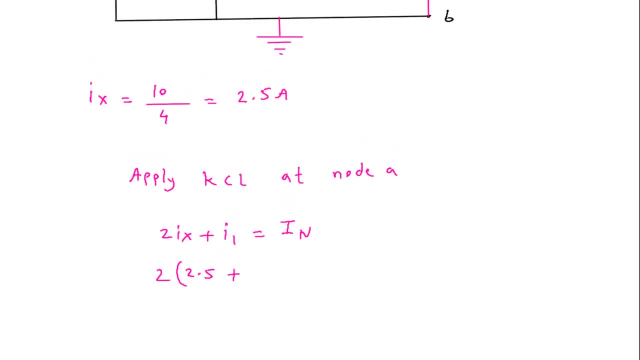 2.5 plus I1 is. I1 is this, I1 is 10, this voltage is 10, so 10 minus 0, because this is connected to ground. so 10 minus 0 by 5, 10 minus 0 by 5 is equal to IN. therefore, 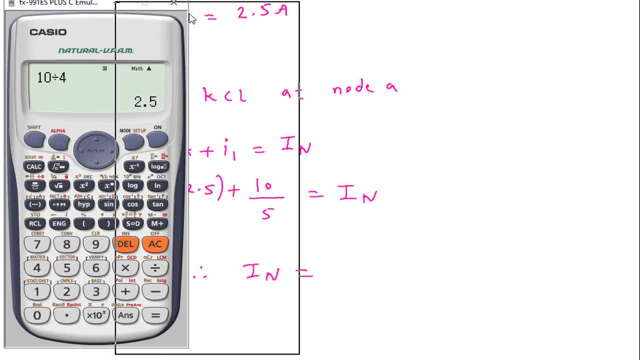 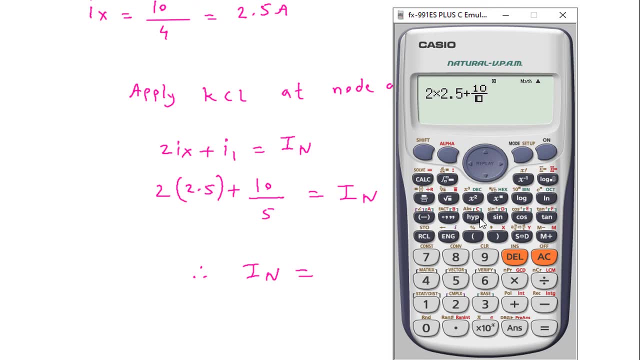 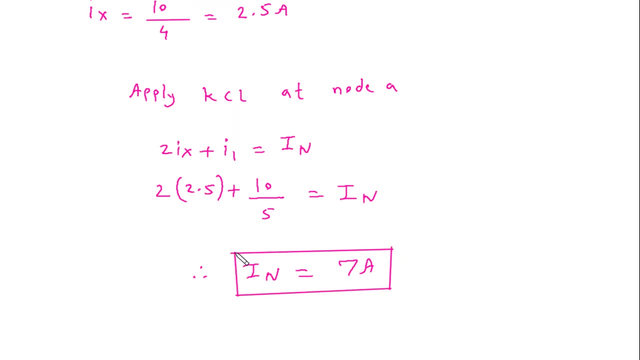 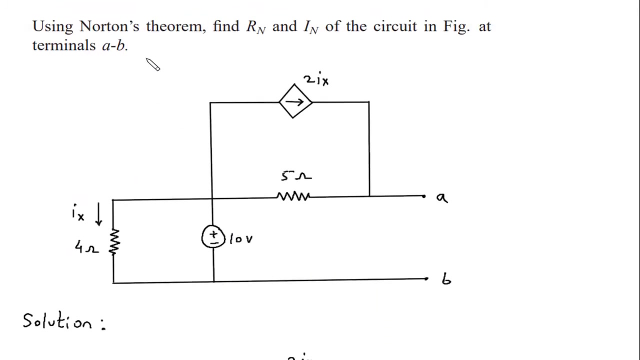 IN is equal to 2 into 2.5 plus 10 by 5, so this is 7 ampere. this is the value of IN, 7 ampere, And Rn is equal to 5 ohm. what we have to find? we have to find Rn and IN, so this: